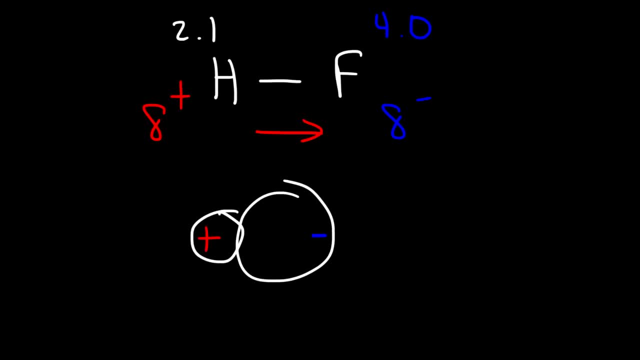 And hydrogen has a positive charge, And so this molecule is polar Because one side is positive and the other side is negative. Now let's make a distinction between polar molecules and nonpolar molecules. In polar molecules, you have an unequal sharing of electrons. 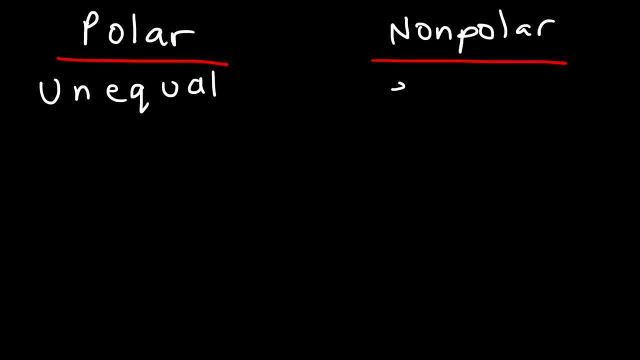 In nonpolar molecules the sharing of electrons is relatively equal. So in the case of hydrofluoric acid, fluorine, even though hydrogen and fluorine are sharing electrons, they don't share equally. So that's why fluorine has a partial negative charge. 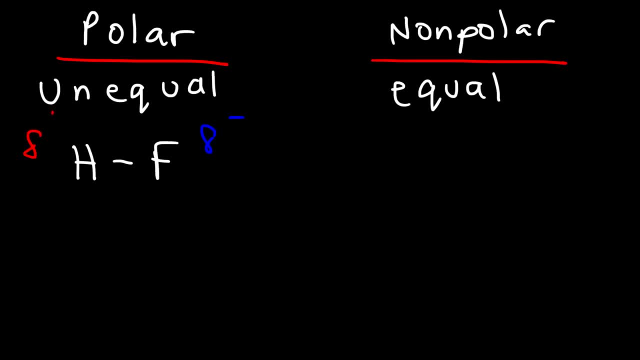 It pulls the electrons toward itself And hydrogen has a partial positive charge. So basically we have this picture: One side is positive and the other side of the molecule is negative. Make an HF polar Hydrogen gas. Hydrogen gas is non-polar. 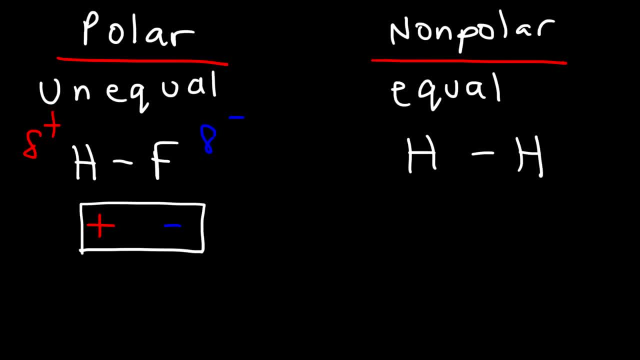 Because the two atoms in the molecule are the same, the electrons are shared equally, And so if you were to draw a picture, you don't have a positive and a negative region. Overall, it's simply just neutral, And so nonpolar molecules. 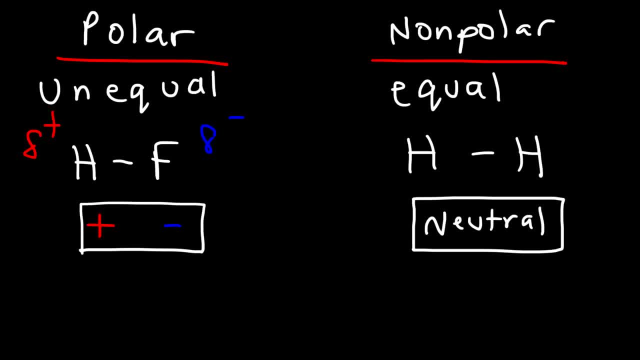 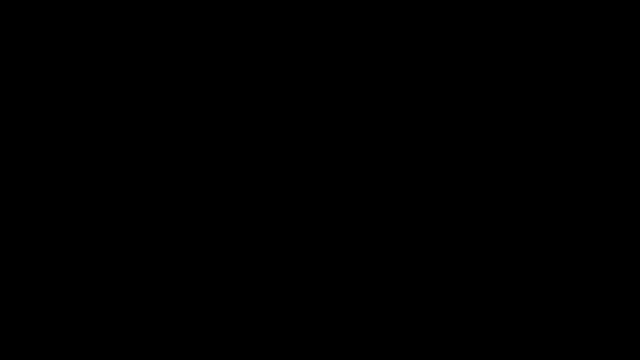 they don't have that separation of charge as we see in polar molecules. So anytime you see a molecule that is made up of one type of element, it's automatically non-polar. So let's go over some rules, Because typically if you're studying for a test, 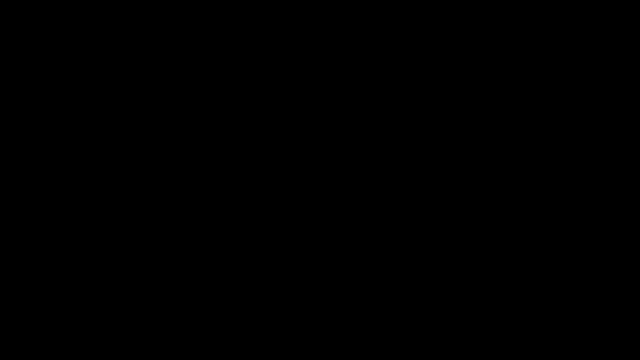 you need to quickly determine if a molecule is polar or not. So let's go over the nonpolar molecules. Molecules that contain only one type of element are automatically nonpolar, such as H2, N2, O2, F2.. 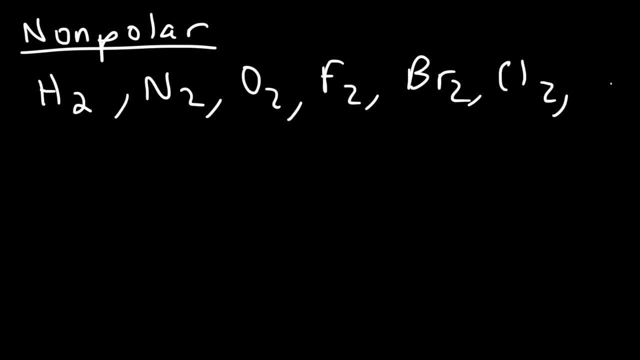 H2, Br2, Cl2, I2.. If you see these automatically, you know it's nonpolar. Now, the second thing you need to watch out for are the hydrocarbons. So if you have a molecule that contains only carbon and hydrogen, 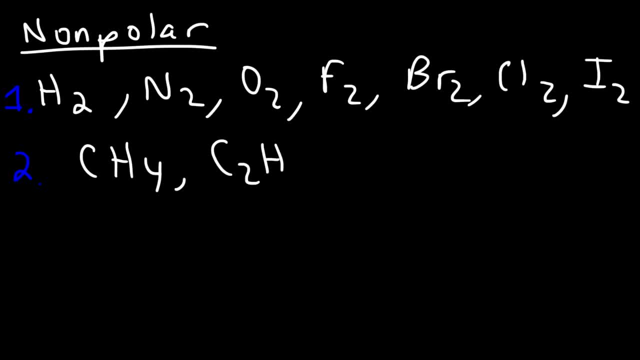 such as methane, ethane, propane and things like that, it's automatically nonpolar. The carbon-hydrogen bond is nonpolar. For a bond to be polar, the electronegativity difference between the two elements in that bond. 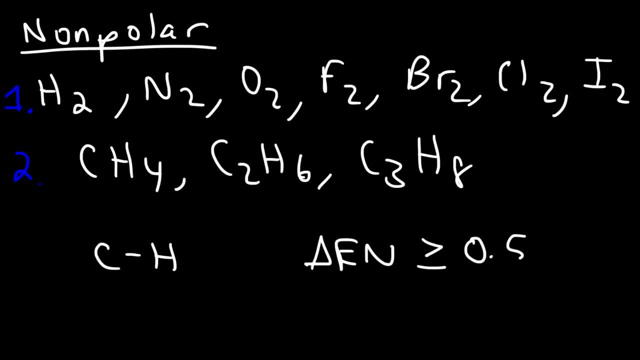 has to be greater than or equal to 0.5 or more. The electronegativity of carbon is about 2.5, and for hydrogen it's 2.1.. So the electronegativity difference between these two elements is 0.4,. 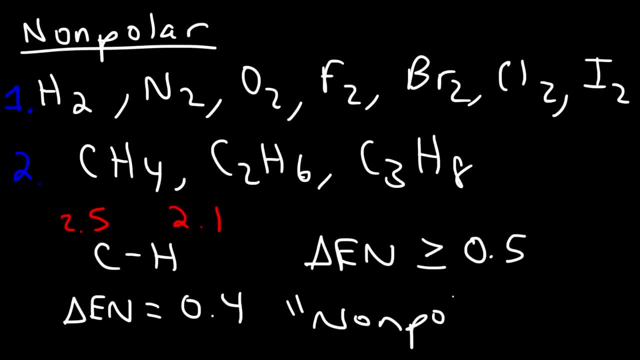 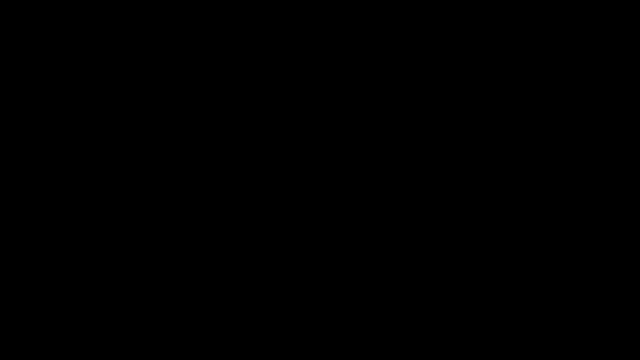 making the bond nonpolar. So hydrocarbons, that is, molecules containing only carbon and hydrogen, are nonpolar. So just by knowing this, this is half the battle. Now, the next thing we need to consider is the geometry of the molecule. 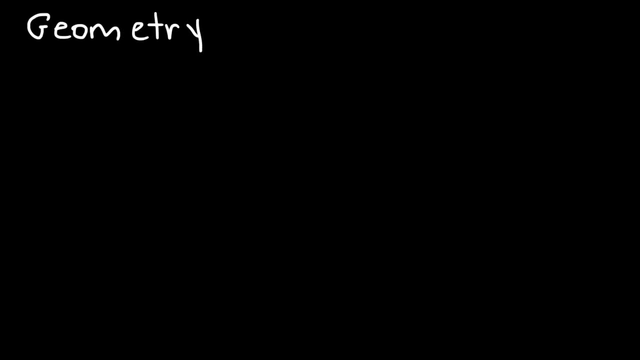 because that could make the difference of the molecule being polar or nonpolar. So let me give you some examples: Carbon tetrafluoride, Would you say. this molecule is polar or is it nonpolar? Well, first, before we analyze the polarity of the molecule, 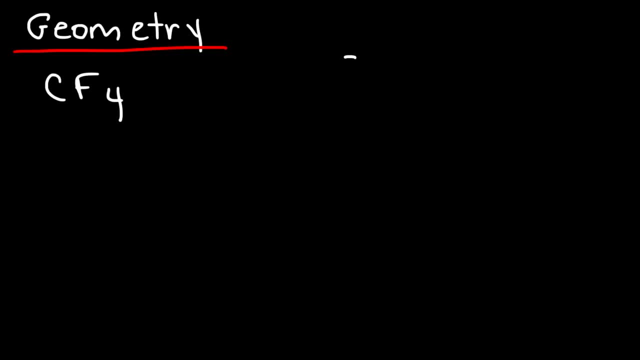 let's talk about the polarity of the bond. Is the carbon-fluorine bond polar or nonpolar? The electronegativity of carbon is 2.5, and for fluorine it's 4.0.. So we have an EN difference of 1.5,. 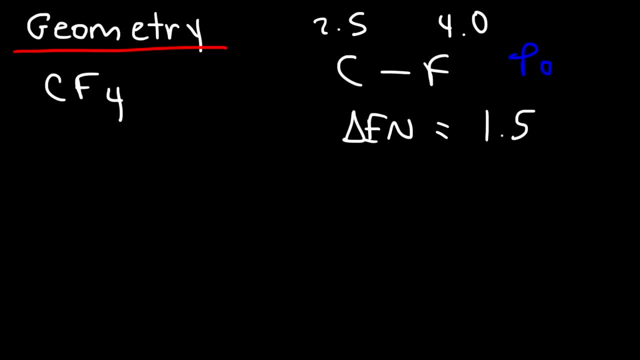 which means that the bond is polar. So not the molecule, but the bond. But now what about the molecule? Is the molecule as a whole? is it a polar or nonpolar molecule? So we need to draw it. So we have four fluorine atoms. 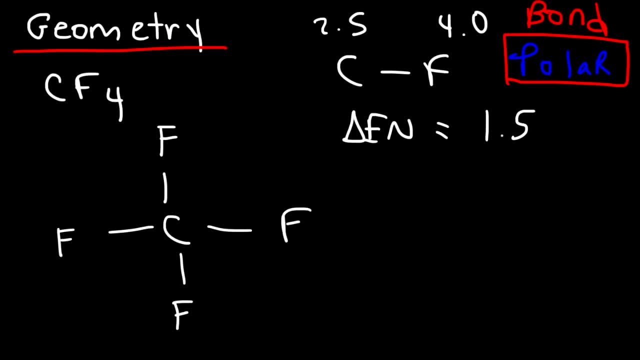 and the molecular geometry for it is tetrahedral, So the bond angles are not 90, but 109.5.. So technically it's a 3D model. It's a 3D shape, not a 2D shape. 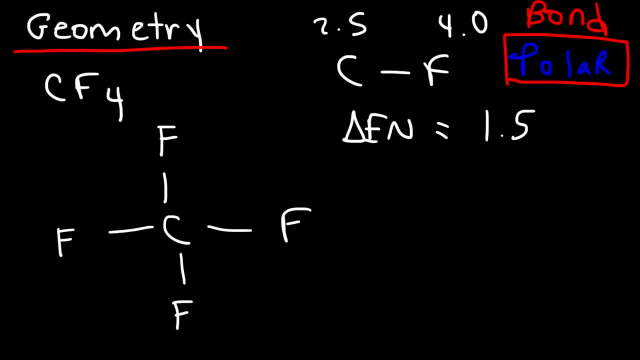 Now you need to draw something known as the dipole moment. The dipole moment looks basically like an arrow that points starting from the atom with the partial positive charge, but it points towards the atom with the partial negative charge, And so the four arrows will look like this. 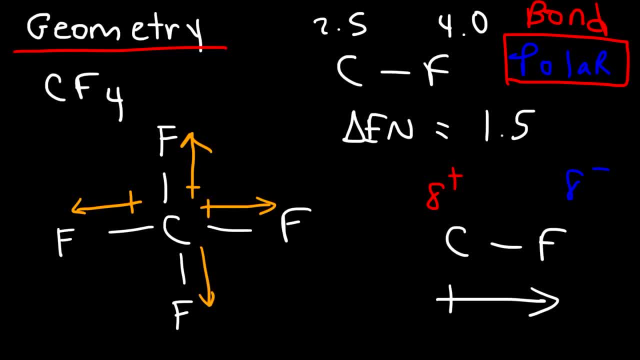 Notice that They all point in opposite directions. These arrows are oriented in such a way that they all cancel out, And so the net dipole moment for this molecule is 0.. So because all of the dipole moments cancel, the molecule as a whole is nonpolar. 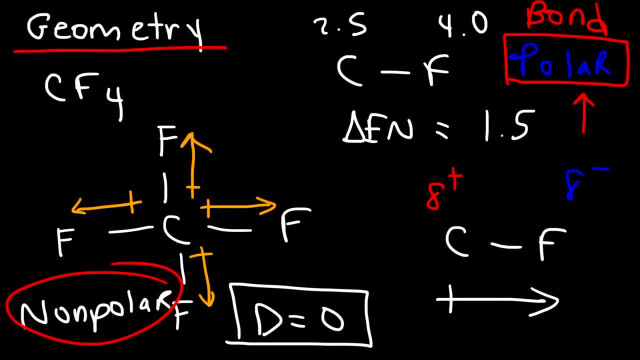 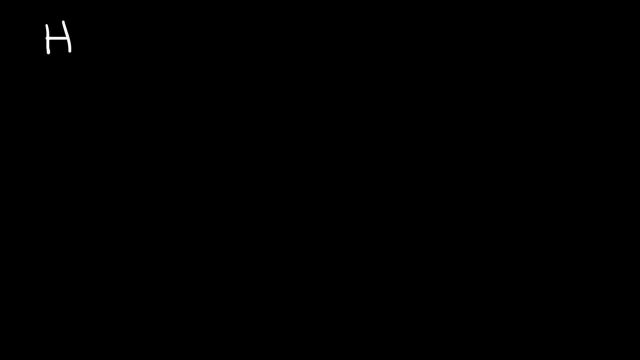 But the bonds in this molecule are polar. So these are things you have to look out for. Now what about water? Is water polar or nonpolar? Well, first let's analyze the bond, the OH bond. Hydrogen has an electron negativity value of 2.1,. 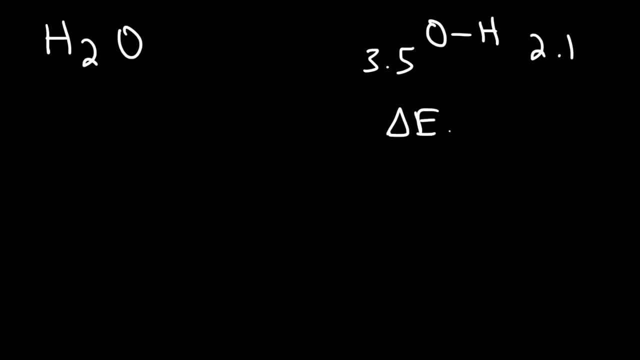 and for oxygen it's 3.5.. So the electron negativity difference is 1.4.. It's greater than 0.5, which means that water has polar bonds. Now we need to analyze the geometry of the bond. 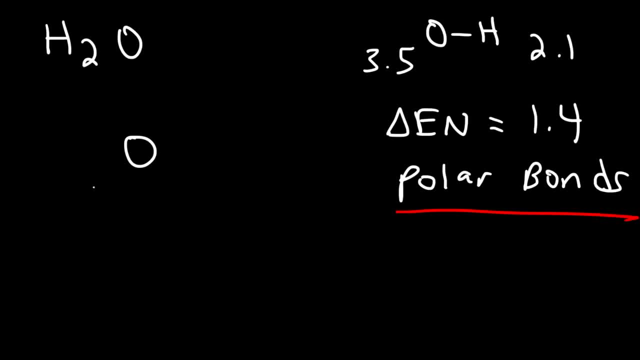 So we're going to look at the geometry of H2O. Oxygen likes to form two bonds and it has two lone pairs And because it's more electronegative, it's going to have a partial negative charge. Hydrogen will have a partial positive charge. 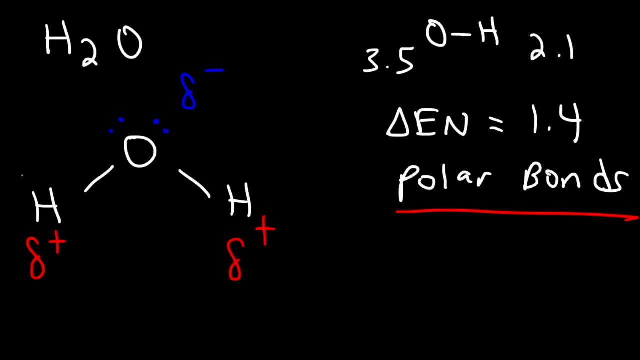 And if we draw the dipole moments, which will point towards the more electronegative oxygen atom, it's going to look like this. So notice that we have a net dipole moment And so, as a result, the molecule is polar. 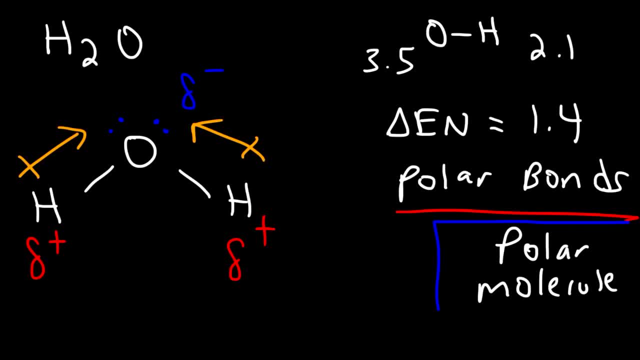 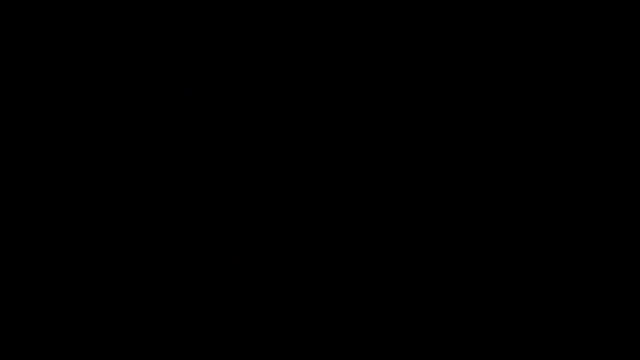 Now let's talk about why the two arrows don't cancel- And hopefully you took a course in physics and you understand how to add vectors. But let's draw two arrows that look like this. Let's call this arrow 1, arrow 2.. 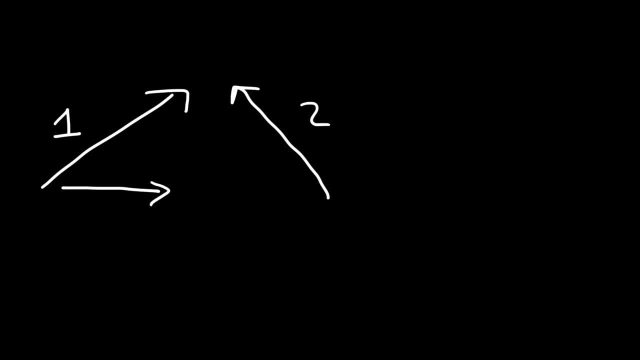 So the first arrow has an X component. The second arrow has an X component that goes towards the right and a Y component that goes up. The second arrow has an X component going to the left and a Y component going up. Notice that the X components they cancel because they're opposite to each other. 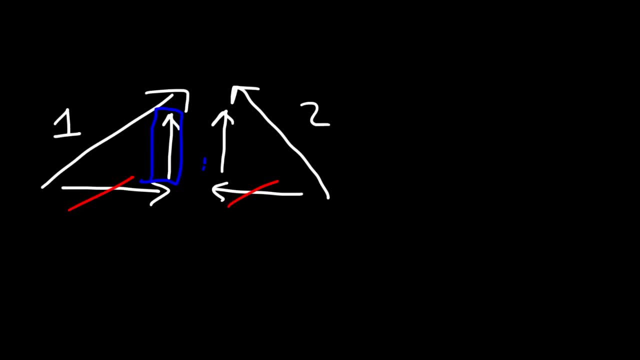 However, the Y components, they don't cancel And so they're additive. Thus water has a net dipole moment that goes towards the oxygen atom. So this side is positive and the top part is it has a partial negative uh charge. 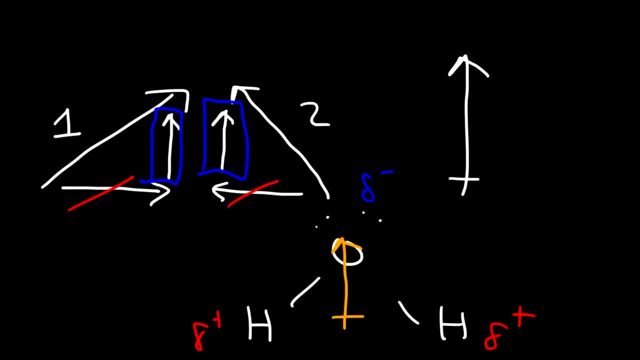 And so the dipole moment goes towards the partial negative oxygen atom making water polar. So molecules that have a net dipole moment are polar, and nonpolar molecules typically have a dipole moment of zero. So keep that in mind. 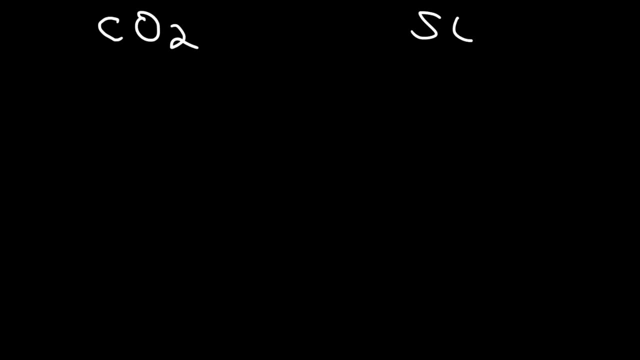 Now let's go over two more examples: Carbon Dioxide and Sulfur Dioxide. Which of these two molecules is polar And which one is nonpolar? Feel free to pause the video and work on this example. Now the best thing to do is to draw the Lewis Structure. 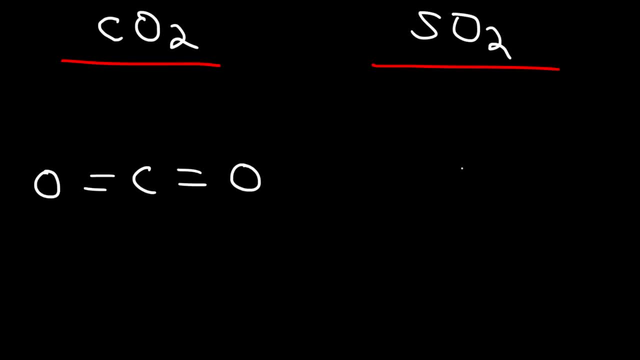 Carbon Dioxide is a linear molecule. Sulfur Dioxide has a bent shape. Now, both carbon and sulfur, they both have an electronegativity value of 2.5.. And we know oxygen has an E-N value of 3.5. 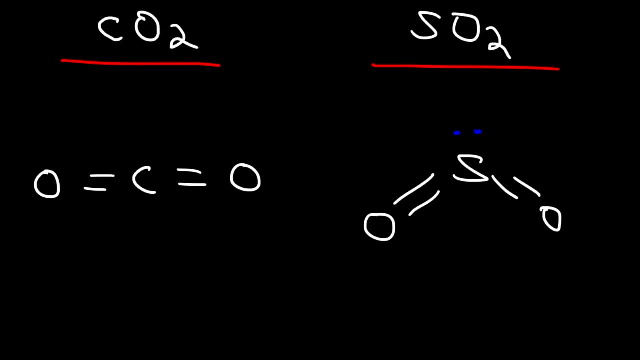 So in both cases, the carbon-oxygen bond and the sulfur-oxygen bond are both polar Because they both contain an E-N difference of 1. So they both have polar bonds. Now let's go back to this example. Now let's draw the partial charges. In both cases, oxygen will carry a negative partial charge, And carbon and sulfur will have a partial positive charge Because they're less electronegative than oxygen. Now let's draw the dipole moments. 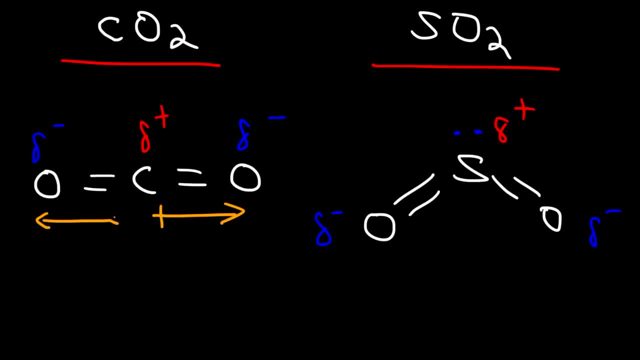 In the case of carbon dioxide, notice that the dipole moments. they're opposite to each other, So they completely cancel. So this has a dipole moment of zero, Which means that CO2 is a non-polar molecule, even though it has polar bonds.